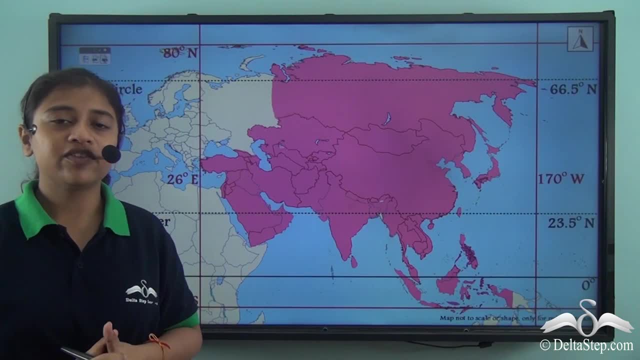 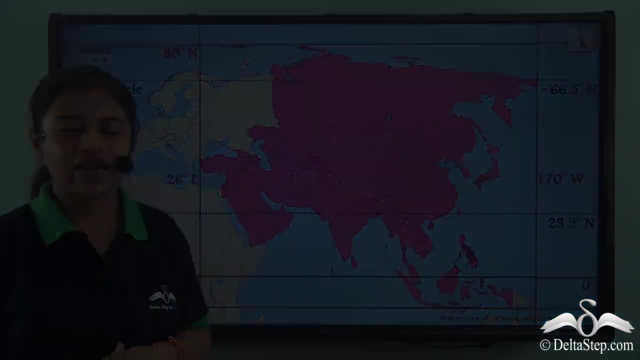 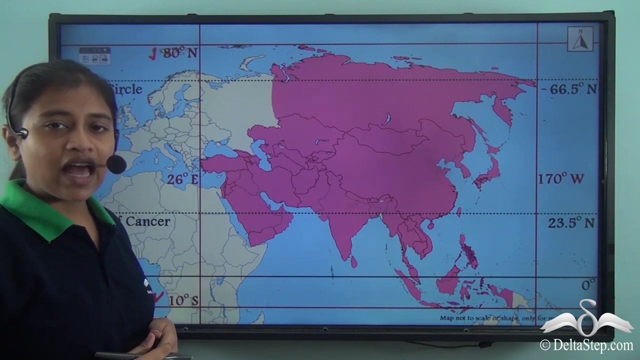 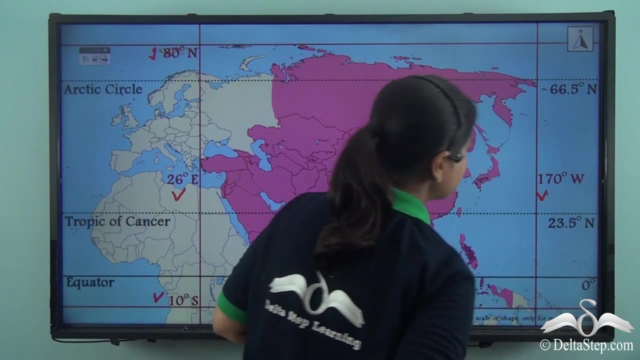 So, as per the map here, we see that Asian continent has a vast latitudinal and longitudinal extent, The latitude ranging from 10 degrees south to 80 degree north and the longitudes ranging from 26 degree east to 170 degree west. So the vast, 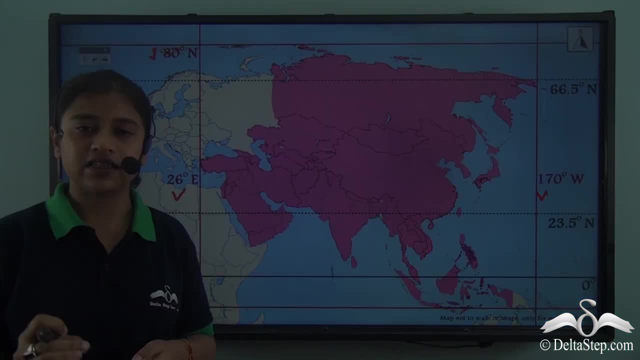 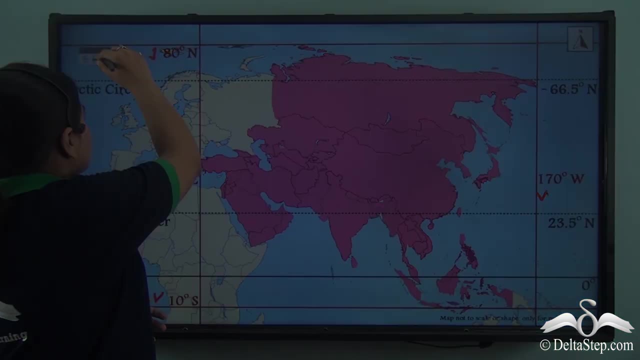 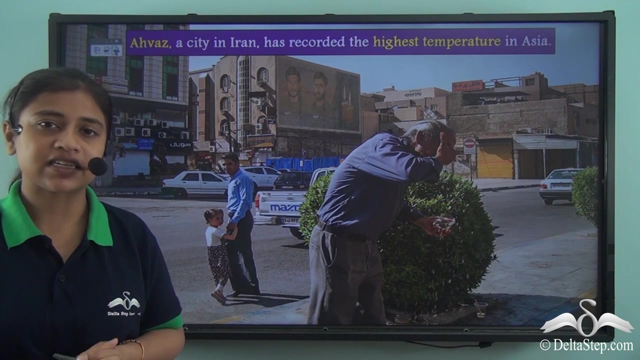 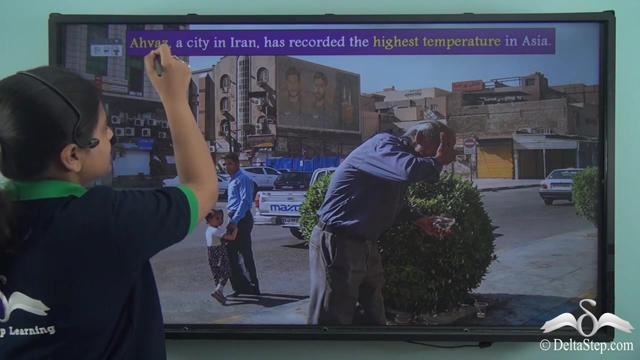 latitudinal and longitudinal extent is the major reason that gives Asia a variety in its climatic conditions too. So, given the point that Asia also has a varied climatic condition, there are certain examples that will help us do so. So Awaz, that is a city in Iran, has recorded the highest temperature in Asia. 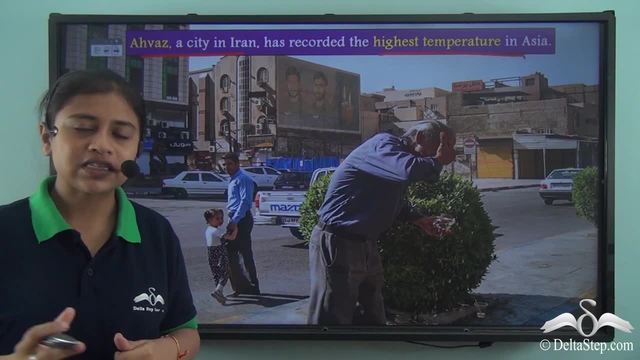 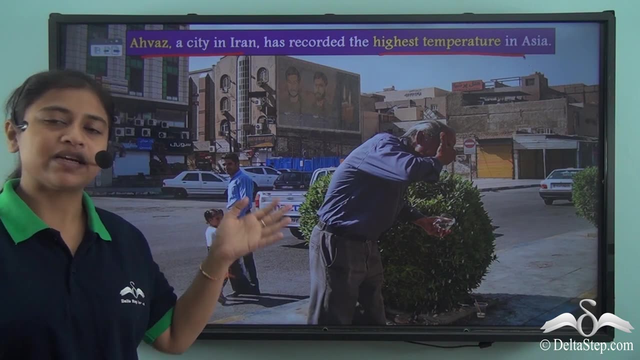 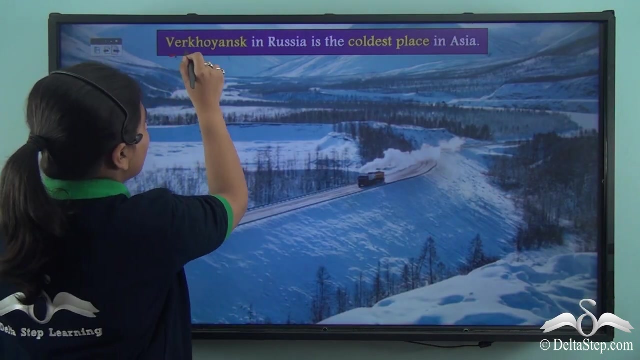 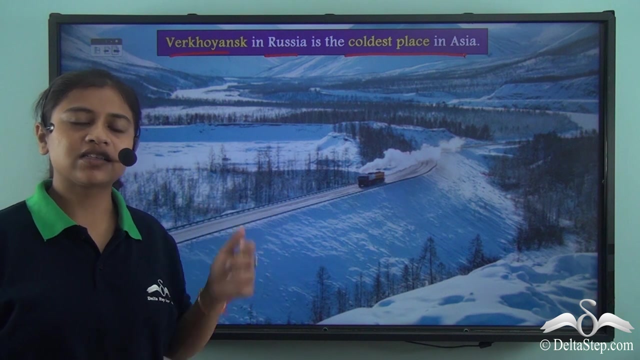 Now Awaz is among one of those cities or one of those places in the world that has recorded the highest temperature, and it is present in the continent of Asia. Similarly, Vero Yanks in Russia is the coldest place in Asia. Vero Yanks is one of those places that are regarded to be the coldest. places on earth, So Vero Yanks in Asia is one of them. Another example is of the wettest place in Asia. Here we are talking about Mohsin Ram. A city in a South Asian country that is, India, is one of the wettest places in Asia. Asia, comprising of one of the wettest places on earth, also is home to one of the driest places on the earth's surface. Here we are addressing to Eden. Eden is a place in Yemen, that is a West Asian country, and it is one of the hottest places on the earth and is a part of the continent of Asia. 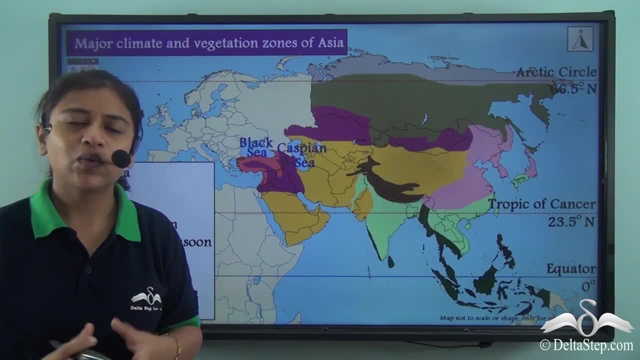 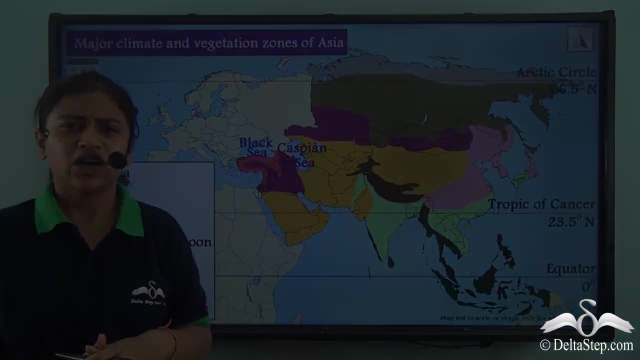 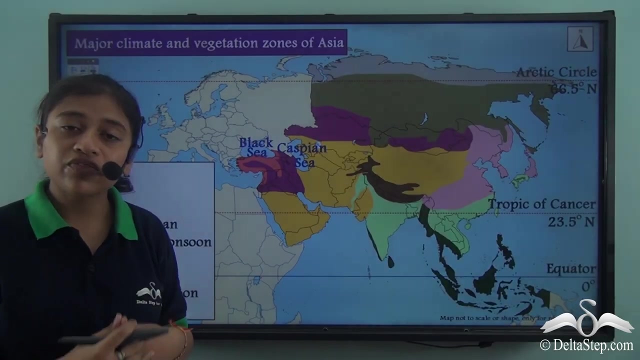 So we just witnessed some places with extreme temperature difference, and they are all present in the continent of Asia. So it must be quite clear by now that Asia has a lot to offer, Not only in terms of the geographical features people cuisine, but also its climatic conditions. 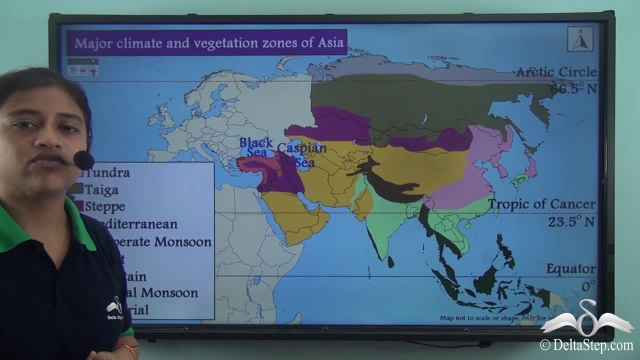 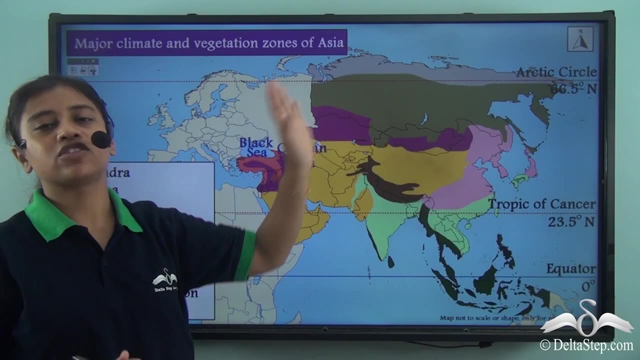 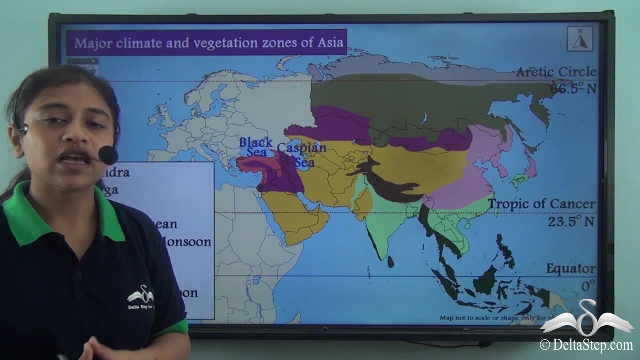 So the vast latitudinal and longitudinal extent of the continent gives it a variety in climatic conditions ranging from the very polar climate type, that is, tundra climate, to equatorial type of climate, So all the climate and vegetation type that falls between these two climate types are all present in the continent. 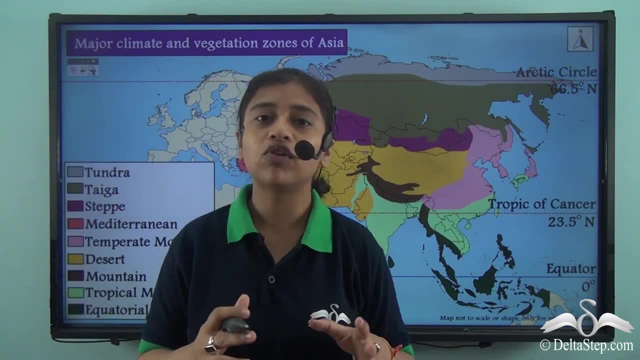 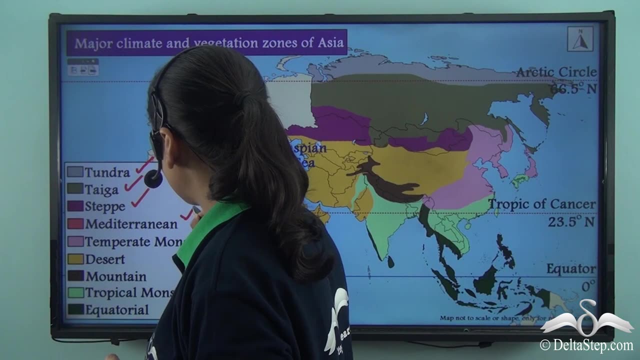 So the major climatic conditions of the continent of Asia are tundra climate, a sugar facilitation, so ficca, meth and others. the boats type of climate is what of the ones are the tundra climate, taiga, steppe, mediterranean and temperate monsoon that fall under the temperate climate? 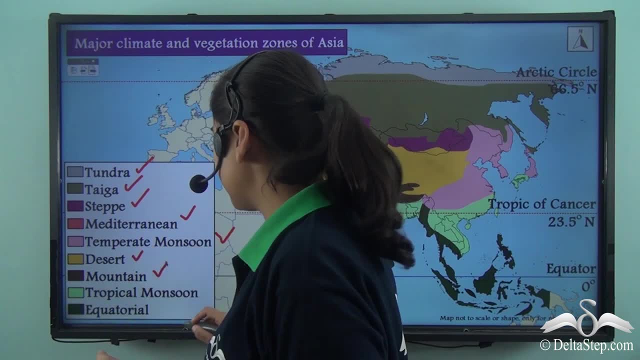 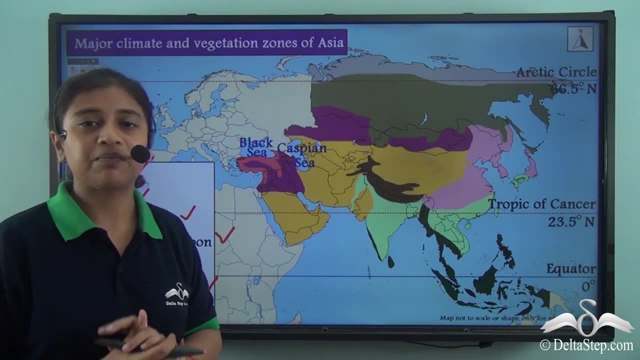 desert climate, mountainous climate, tropical, monsoon and finally, equatorial. So all these climatic conditions that prevail over the continent of Asia has its subsequent vegetation type, confirmed by E诸 WES rounds. So all these climatic conditions that prevail over the continent of Asia has its subsequent vegetation type, 1-2, as seen here. 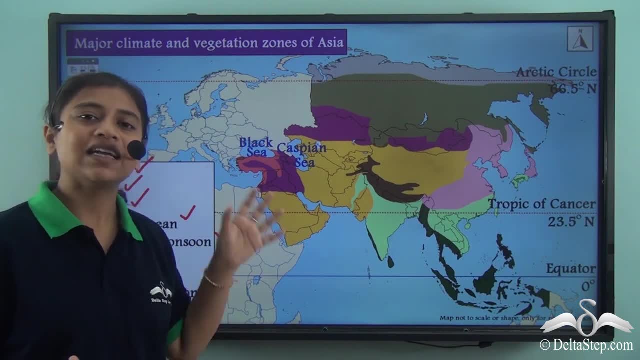 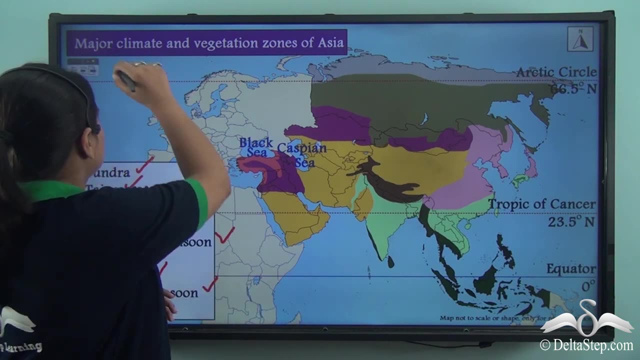 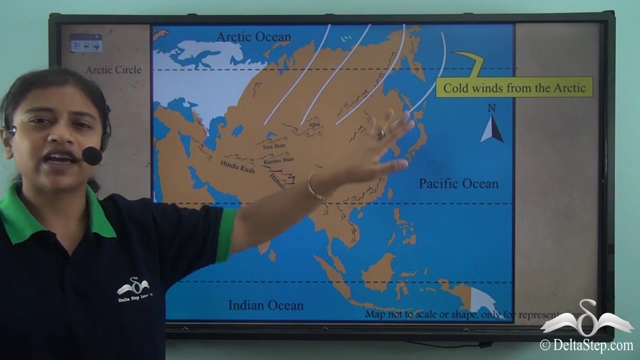 and wildlife. So we will be taking a look at each of these climate conditions, their vegetation and wildlife one by one. Cold, chilly arctic winds blow from the northern part of the continent to the central regions. They blow down unchecked, giving the central portion 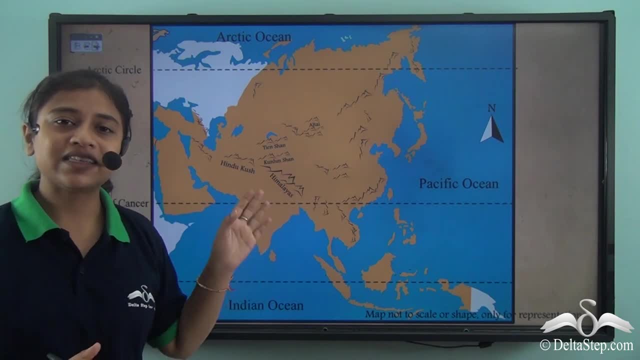 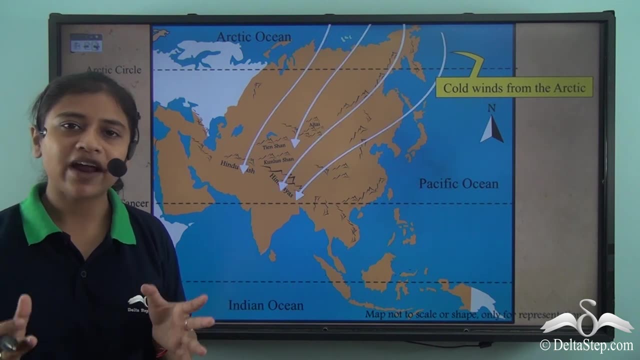 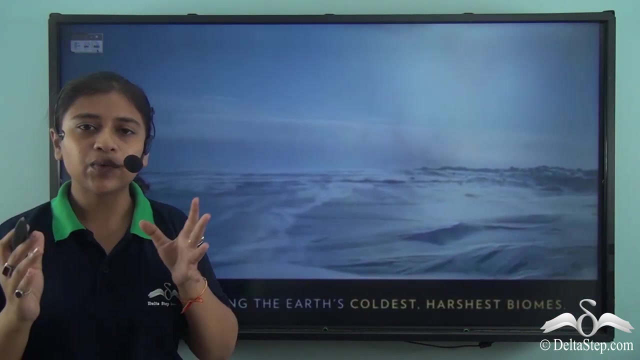 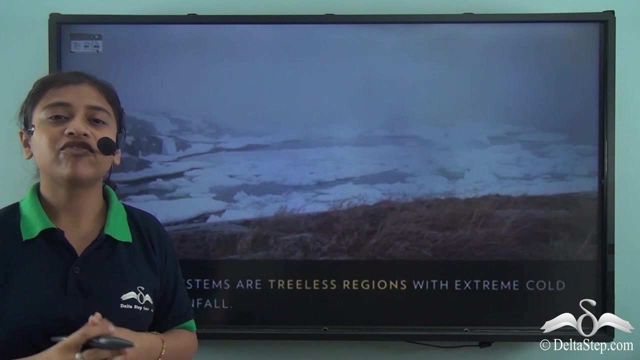 of the continent, severe winters, while the central and eastern portion of the continent has mountain ranges that act as barrier to this chilly winds. So because of that arctic wind and the severe winters that span over the northern part or the central part of the continent, here we have the tundra biome. So tundra biome is believed to be the harshest. 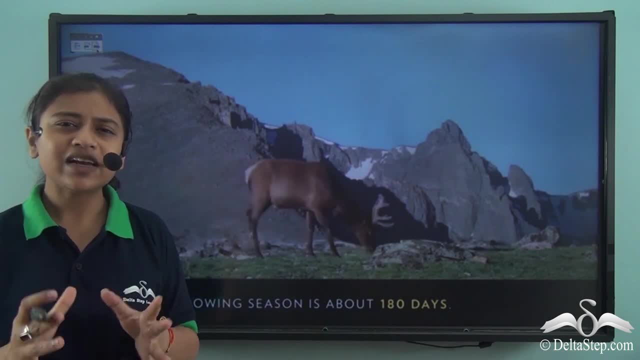 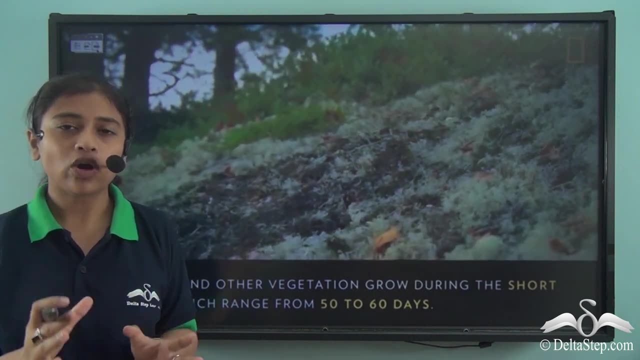 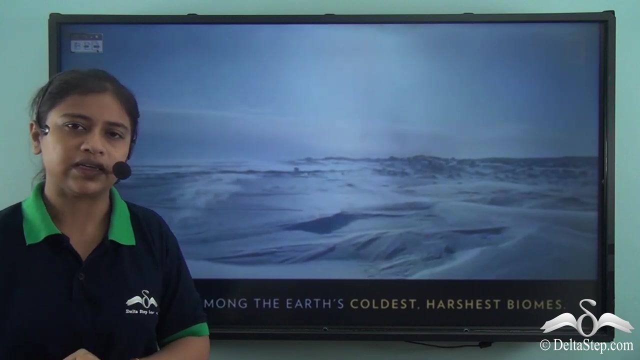 and the coldest biome of the world, With treeless regions, low rainfall and severe winters. the growing season is very less, with short shrubs and vegetation in the summer season that is very short, ranging upto 50 to 60 days only. So in the very short summer that is present, 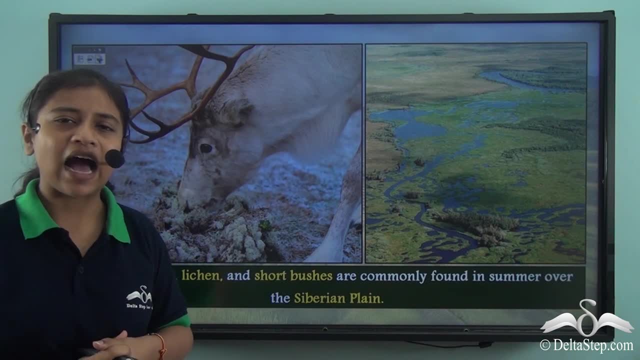 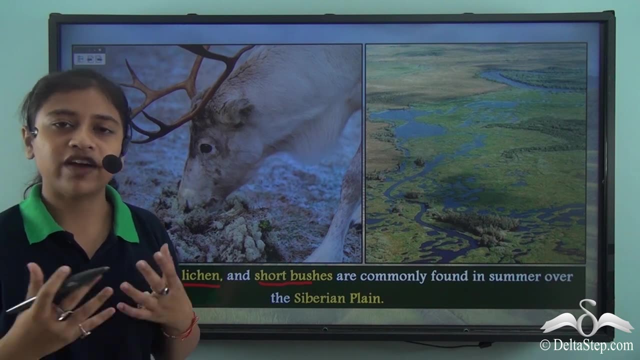 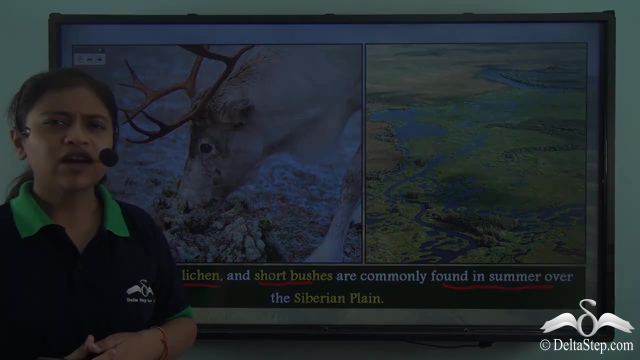 or that is prevalent over the Siberian plain. we have reindeer moss, lichen and short bushes, part of the vegetation that grows or are found in the summer season over the Siberian plain. Now can you guess why do we call the moss over the Siberian plain? 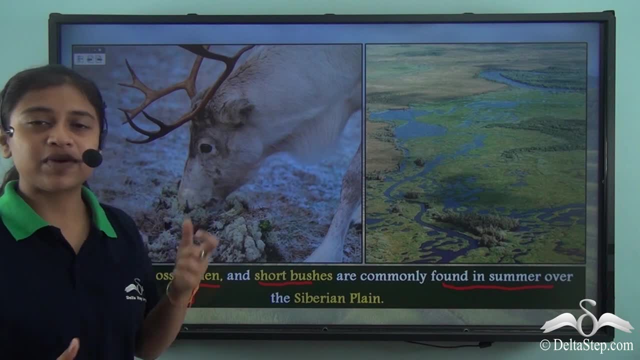 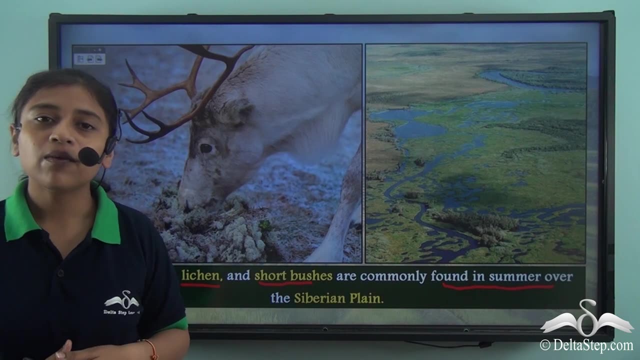 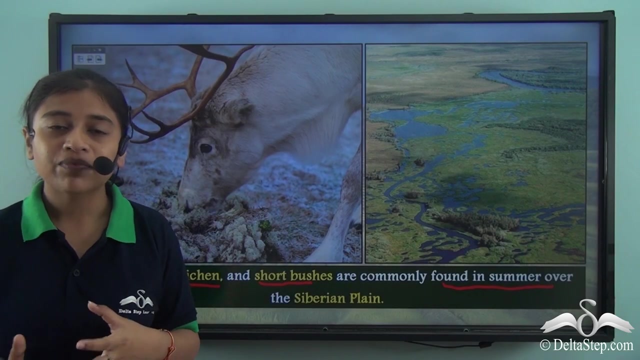 the reindeer moss, because Santa's reindeer that are present in this region gobble up the reindeer moss and they enjoying eating this vegetation. So the Siberian plain in the northern part of the continent experiences a tundra type of climate and here the vegetation is very less, with low rainfall and severe 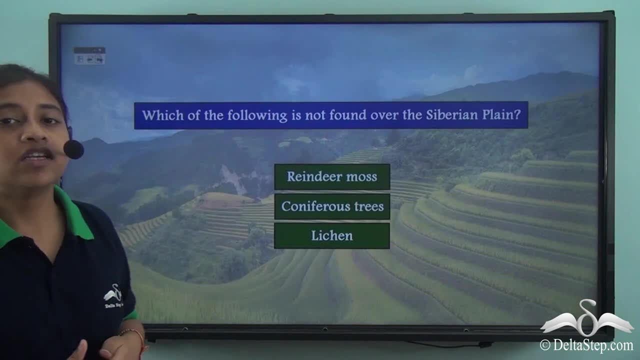 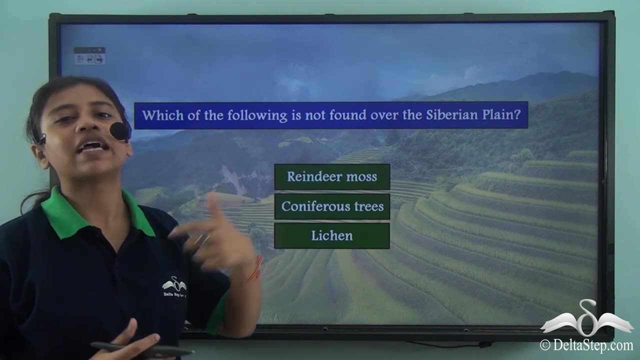 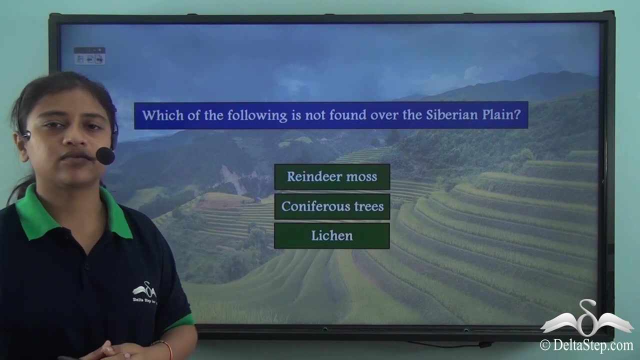 winters. So before we proceed with the lesson, could you help me answer this simple question: which of the following is not found over the Siberian plain? is it the reindeer moss, the coniferous trees or the lichen? Yes, the correct answer is the coniferous trees. 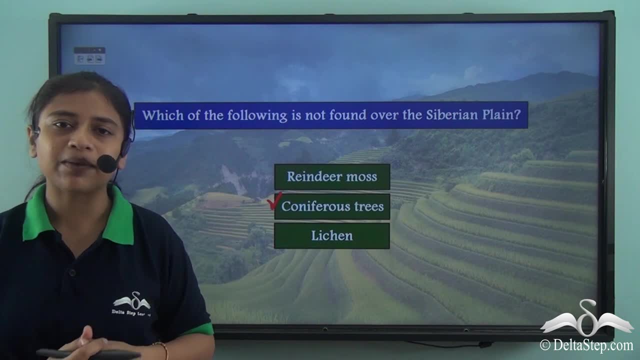 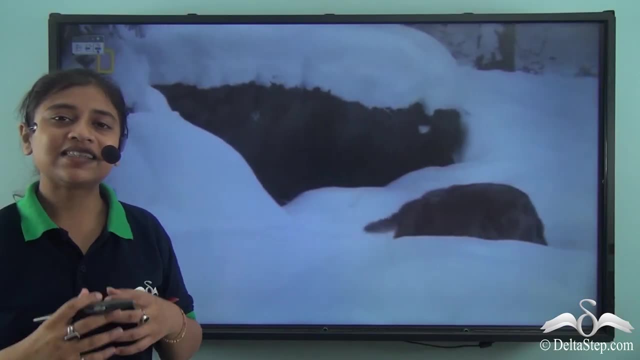 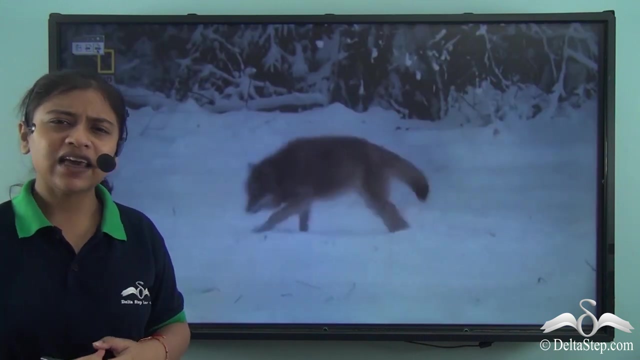 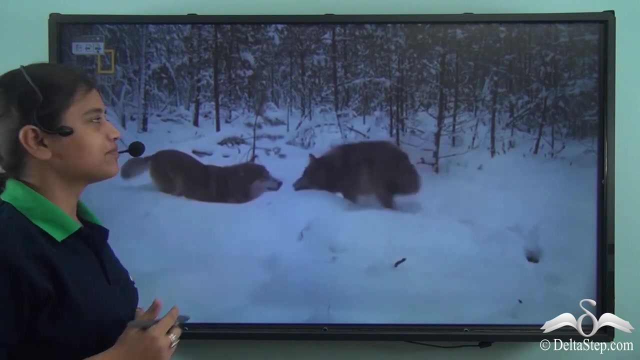 While reindeer, moss and lichen is found over the Siberian plain, coniferous trees are not found here. Besides Santa's reindeer, we also find Polar Dogs over the Siberian plain, and they have adapted themselves to the extreme cold conditions and live here happily, as you see. So in this lesson we were able to understand. 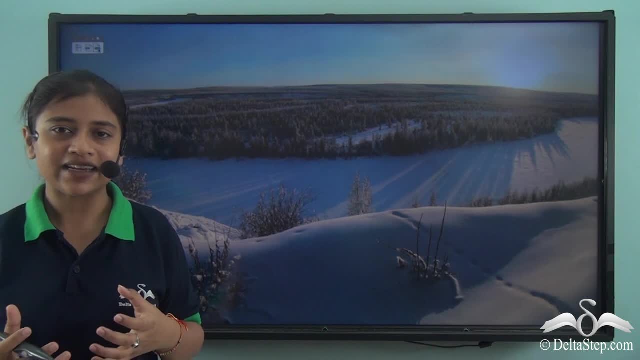 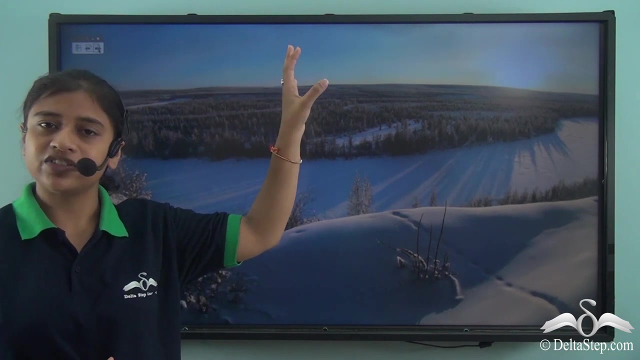 that the vast longitudinal and latitudinal extent of the continent of Asia gives it a variety even in its climatic conditions. We saw that the climatic conditions of the continent ranges from the tundra type of climate in the very north, near the Arctic region, to the 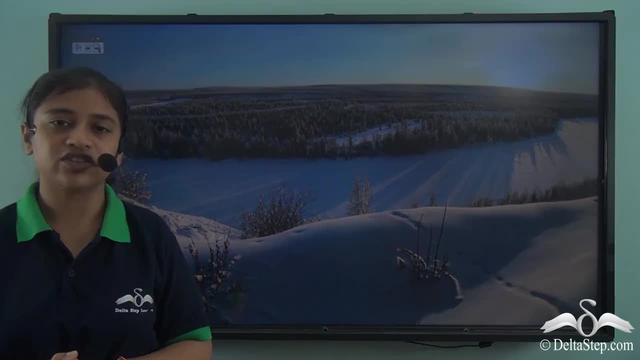 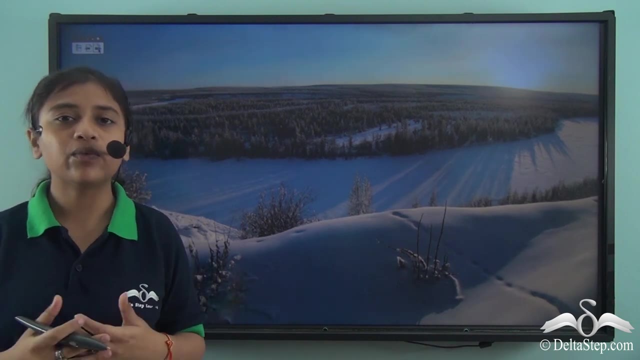 equatorial type of climate over the equatorial region. So in this lesson we learnt about the tundra type of climate, the vegetation that is found there and also the wildlife. In our next lesson we will be taking a look at other climatic conditions and the respective 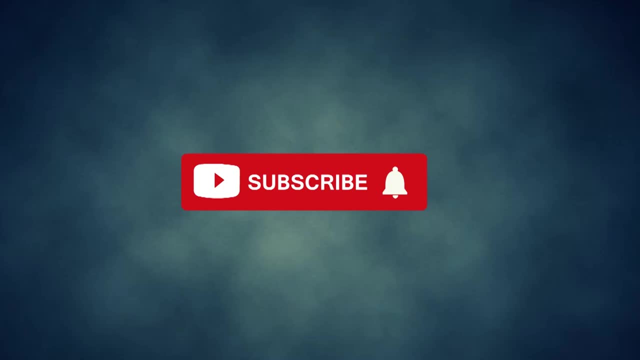 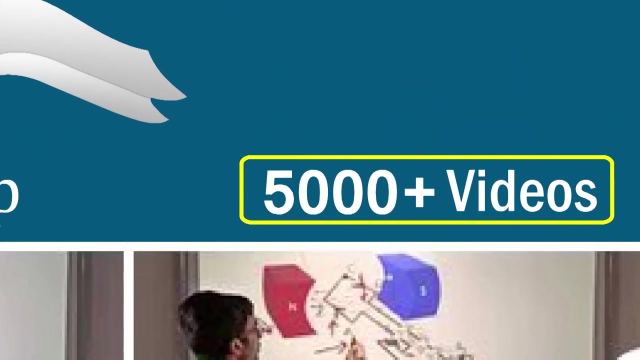 vegetation and wildlife. Don't forget to subscribe to our channel and hit the bell icon. You can also register for free at Deltastepcom or download the Deltastep app to learn one to one with our amazing teachers or to get access to all our free lessons.